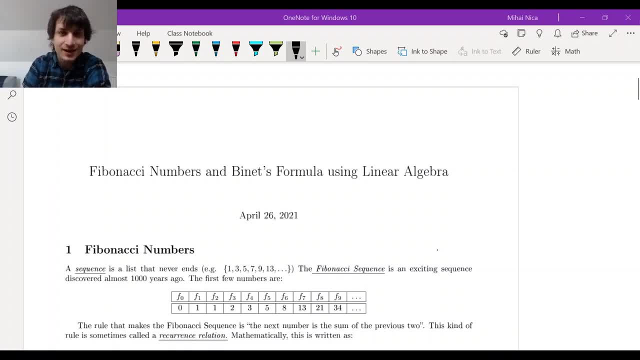 Hello, In this video I'll be going over the Fibonacci numbers using linear algebra. So linear algebra is a very general set of tools that you can use for almost anything, And I'm gonna make the Fibonacci numbers fit into that framework. And what I want to get to is something called Binet's formula. 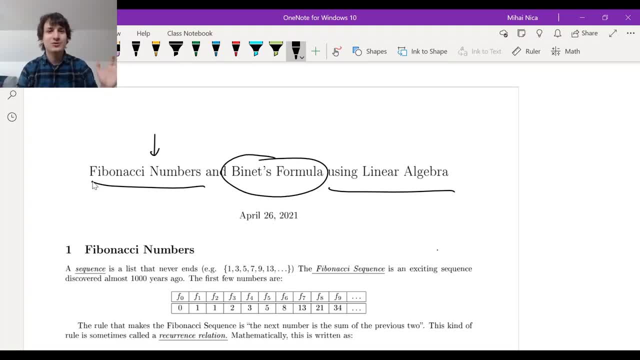 and that is an explicit formula for the Fibonacci numbers. So what I want to show you is how you can use linear algebra to get this formula, how you would discover the formula. So, that being said, there will be some linear algebra background, so if you've never seen matrix multiplication before, this video probably won't make a lot of sense. 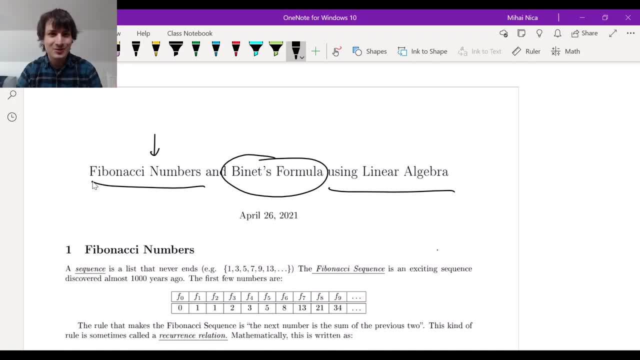 But if you have seen matrix multiplication, then I think there's some useful knowledge you can get out of it, And I think it's a really cool application of linear algebra. Okay, so here we go. We're gonna start with. what are the Fibonacci numbers? 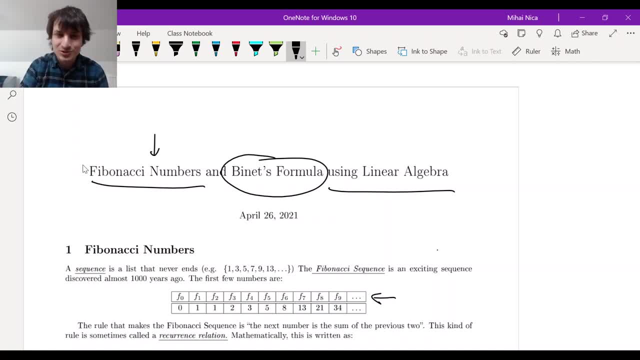 And there are this sequence of numbers: It starts with 1, 1.. So I call the numbers f1, f2, f3.. So the first number, f1, is 1.. The second number, f2, is also 1.. It starts with 1, 1.. 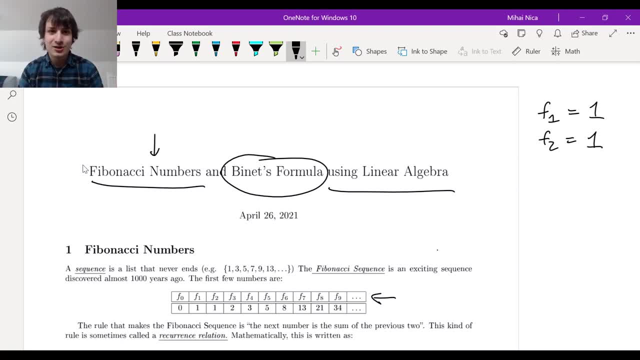 And the next number is always the sum of the previous numbers. So the third number, f3, is 1 plus 1. That's 2.. The fourth number is 1 plus 2. That's 3.. The fifth number is 2 plus 3. That's 5.. 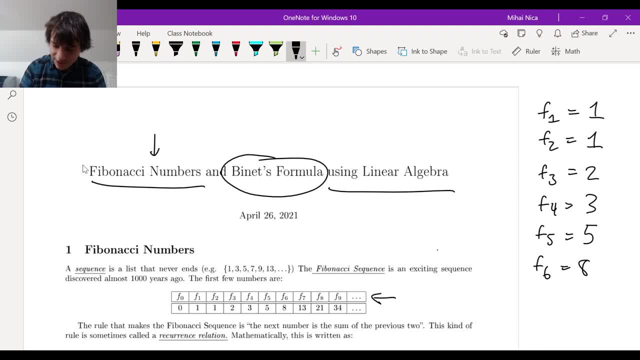 The sixth number, f6, is 3 plus 5.. That's 8. And so on and so on. And to be inclusive, to include people who like to start at 0,, we're also going to make f0 equal to 0.. 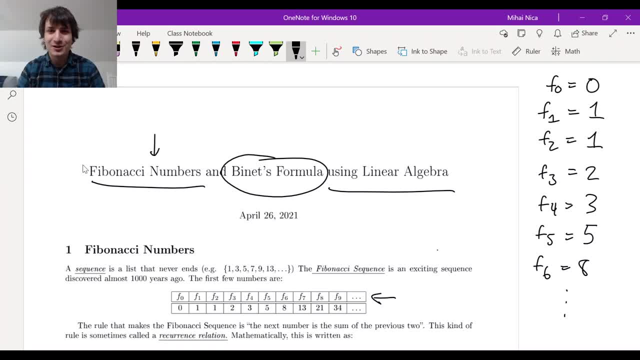 And that just continues the pattern, but starts at 0 instead of starting at 1.. So here's a list of all the numbers: 0, 1,, 1,, 2,, 3,, 5,, 8,, 13,, 21,, 34.. 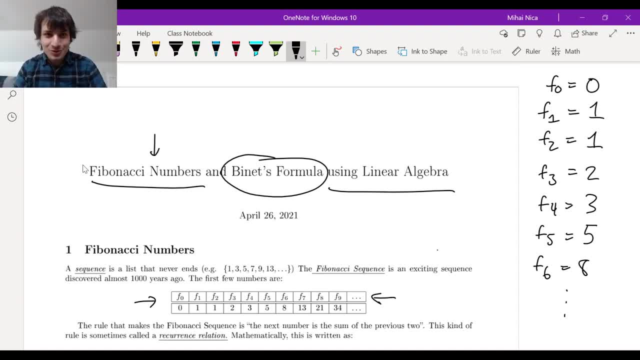 And you could go forever and ever. And the issue you might have with the Fibonacci numbers is that to calculate the 100th Fibonacci number- like f100, you might think, oh well, that's going to be a lot of work. 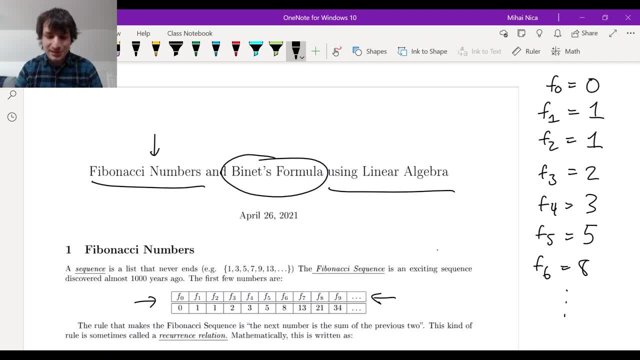 We're going to have to add numbers until we get up to 100. But it turns out there is an explicit formula. So this formula is called Binet's formula And it looks like this. So it has some nasty things in it. 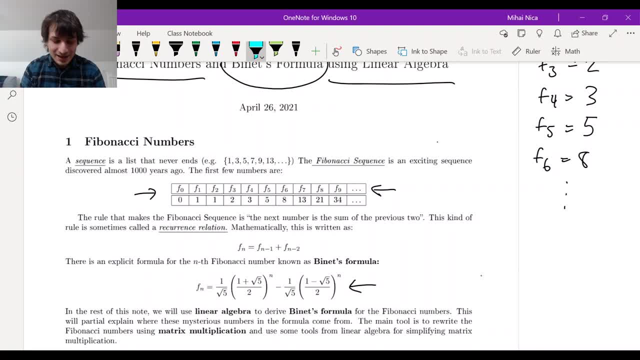 Let me write out what it is. So fn, that's the nth Fibonacci number, And you can get it just as a function of n, So you don't need to calculate anything else, No sums or anything- And what you do is you take this number. 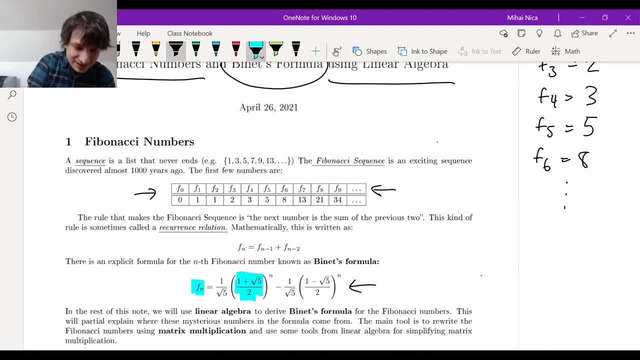 1 plus square root of 5 divided by 2, and you take that to the power n. You take that to the power n. Then you take 1 minus square root of 5 divided by 2, and you multiply that to the power n. 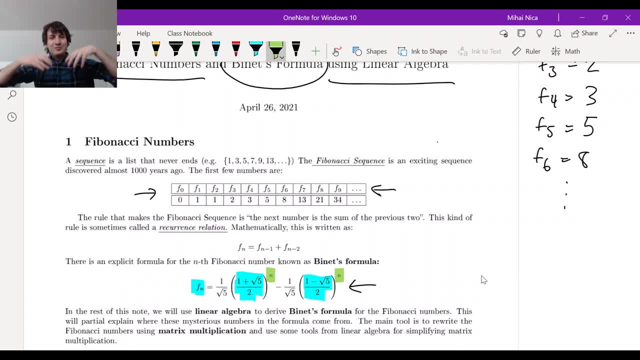 So these are two crazy, irrational numbers with square root of 5.. You take them to the power n, You multiply them by this funny factor of 1 over square root of 5. And you subtract them from each other and that gives you the nth Fibonacci number. 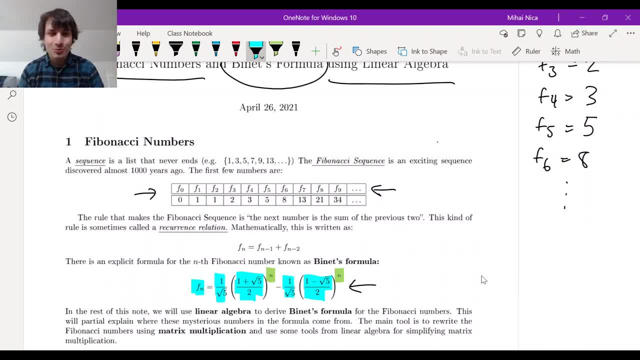 So this is Binet's formula. It's been known for a long time, And what I want to do in the rest of the video is use linear algebra to explain where this comes from. So you know these numbers. you might say like: 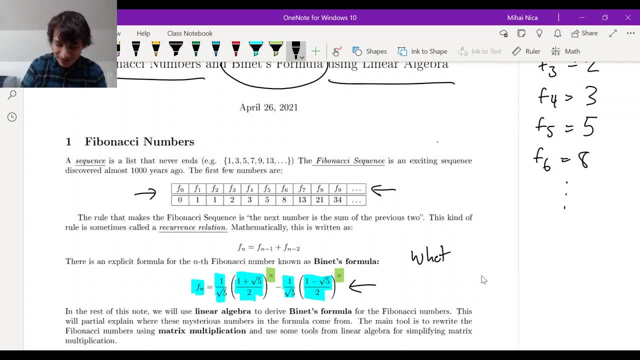 where are these numbers coming from? What is going on here? So I'm going to try to explain that using linear algebra. Okay, so that's what we're going to do, And the first thing we're going to do is we're going to convert the Fibonacci numbers. 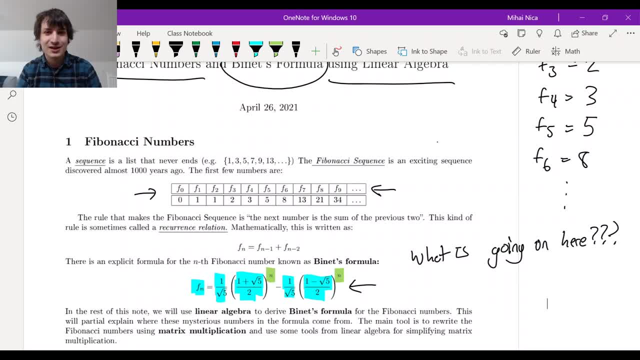 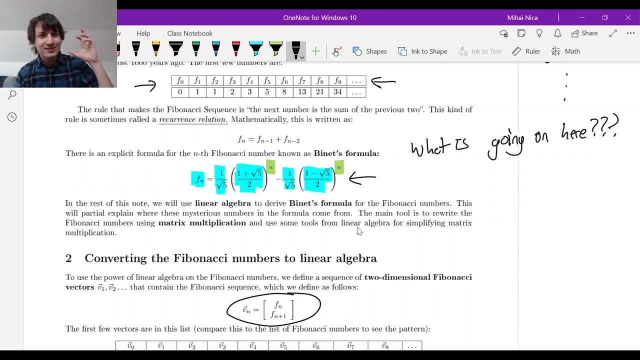 from a sequence of numbers into a sequence of vectors. So I'm going to define these Fibonacci vectors. So there's going to be Vn And the rule is you just take the Fibonacci number n and the Fibonacci number n plus 1, and you put them in a vector. 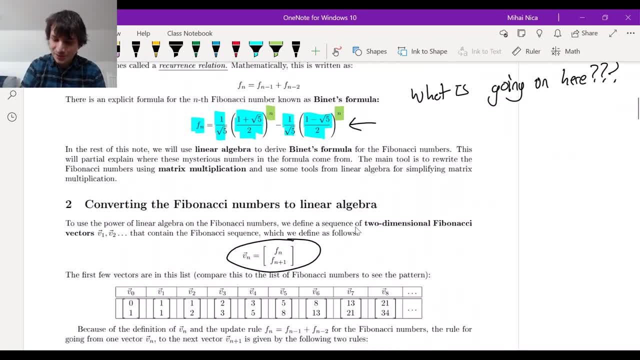 So here is a list of all the vectors so you can see what's going on. So remember, F1 was equal to 1 and F2 is equal to 1.. So that means that the first vector- V1, is just 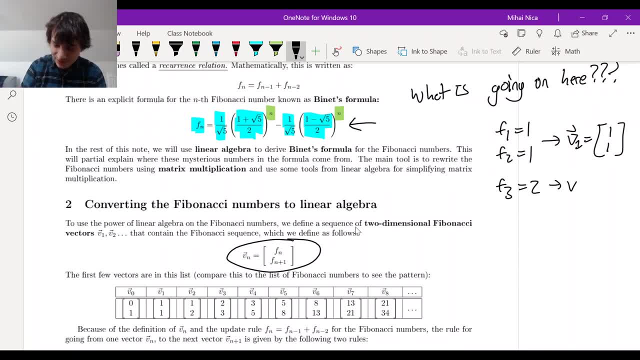 And the next Fibonacci number is 2.. So that means the next vector, V2, is, And so on. So you take the Fibonacci numbers and you just stack them up. Maybe it's helpful to sort of have these both in the same frame. 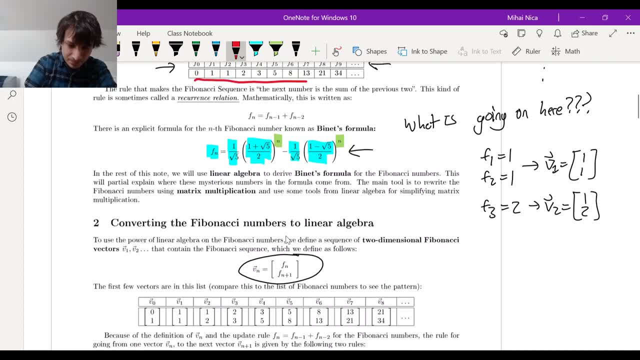 Let's zoom out a bit So you can see the Fibonacci numbers up here. And here are the vectors, And what we're doing is we're just stacking two consecutive Fibonacci numbers into each vector Vn. That's how I made the vectors Vn. 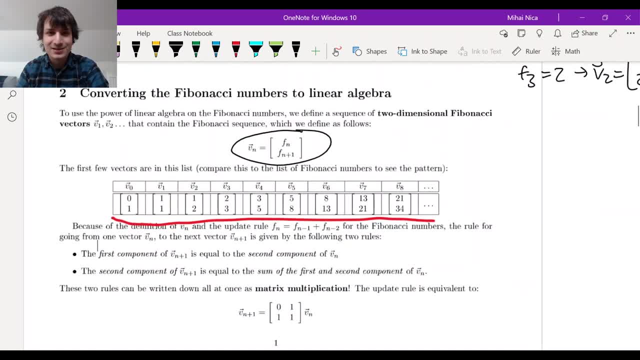 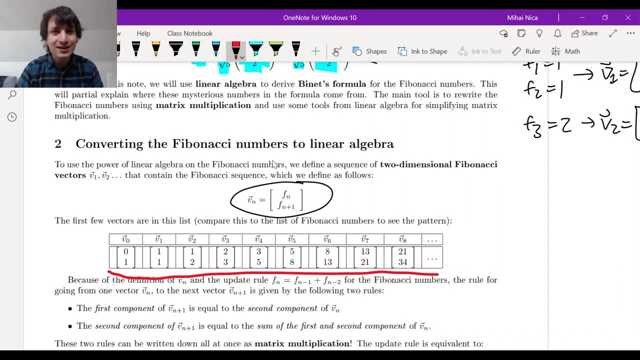 So why on earth would we define the vectors Vn like that? So the reason is that, because of the rule for getting from one Fibonacci number to the next Fibonacci number, the definition of the vector Vn- the Vn's have a very nice rule with matrix multiplication. 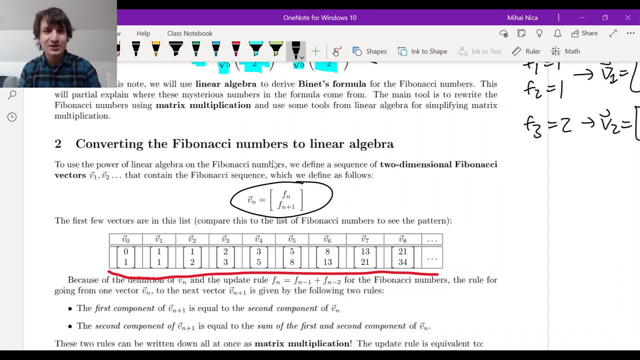 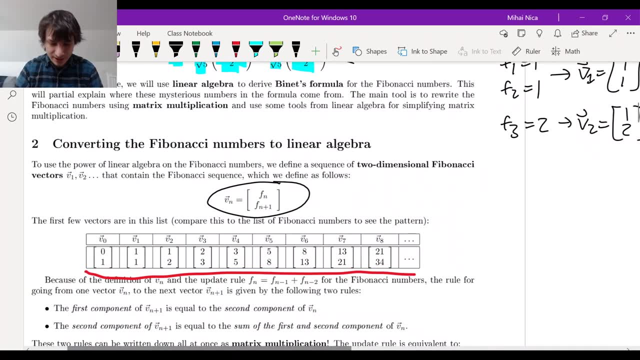 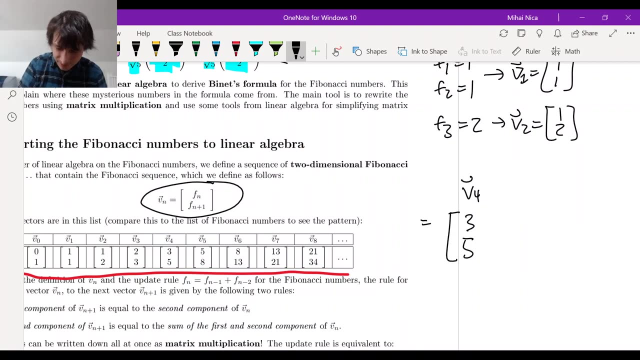 So let's see what that rule is. So here are the two rules to go from one vector V to the next vector in the sequence V. So let's do it as an example. Let's start with V4.. So V4 is the vector. 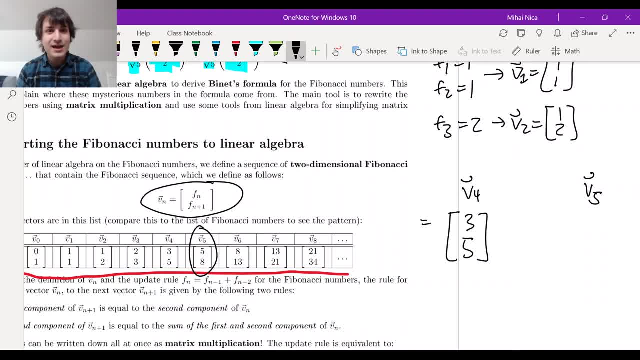 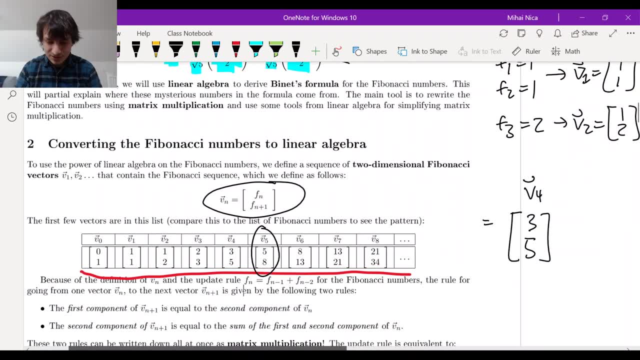 And we know that V5, here it's, on the sequence it's, but let's see how you would get the vector, the vector, And there are two rules that tell you what to do. So the first rule is that the first component of the next V in the sequence 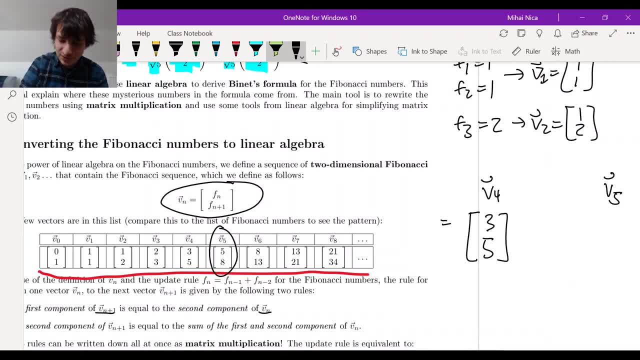 is given by the second component of Vn. So the first thing you do is you take this 5 down here and you put it in the first component of V5.. So you get 5 up here, So that sort of just gets copied over. 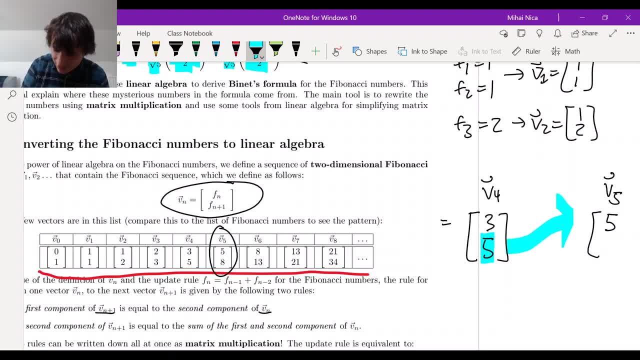 Let's just draw a little copy arrow, like that. It gets copied over like this: That is the first thing you do to make V5.. You copy over the 5, the bottom component. What's the next thing you do? Let's get rid of this highlighting here. 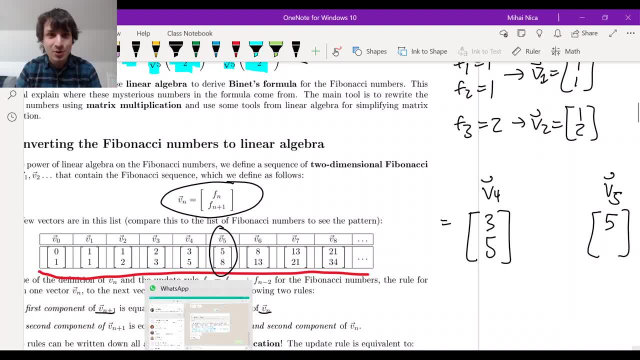 The next thing you do- and this is the second rule- the second component of Vn plus 1 is equal to the sum of the first and second component of Vn. So now, what we're going to do is we're going to take the 3 and the 5,. 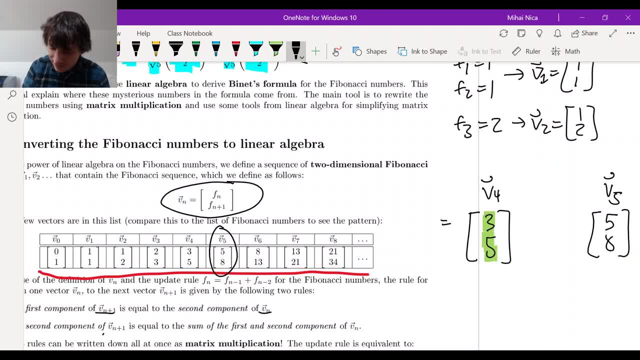 we're going to add them together. that gives you an 8, and you put that in the second component, And this is just because of the Fibonacci rule. So the Fibonacci rule says, to get the next Fibonacci number, you do the sum of these two. 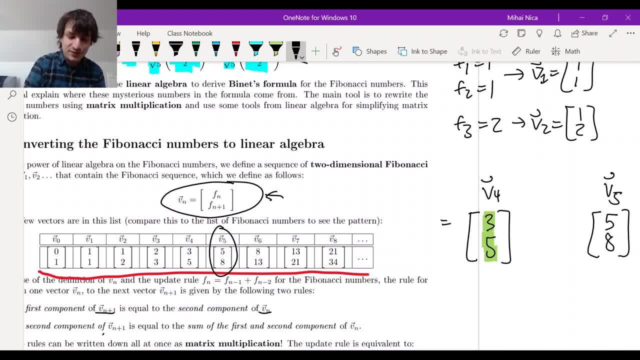 and that's exactly what's going on. So if you look at the definition of the Vn's and the Fibonacci number is Fn, we're just copying down what the rules are. So that's how you go from one vector- V4- to the next vector, V5,. 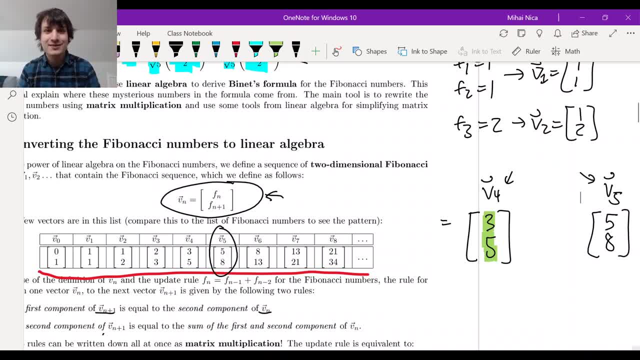 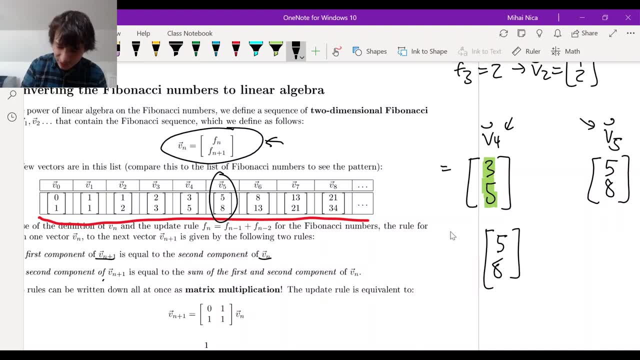 and it works in general. And the nice thing about these rules is that they are linear. So another way to describe what we just did is you could describe it like this: You could say that 5, 8, that's the vector V5. 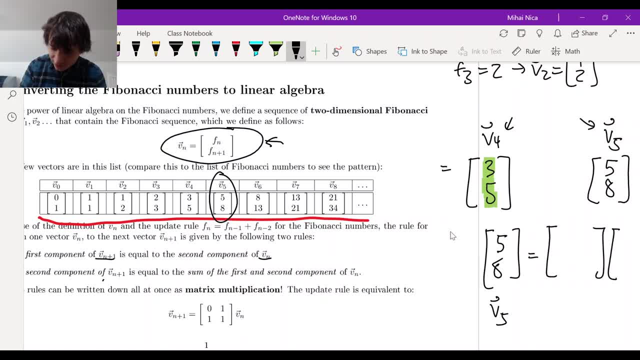 This is a matrix multiplication. This is a matrix multiplication times the vector 3, 5.. Okay, which matrix multiplication is it? We want 0 copies in the first column. So in the first column, that's these two coefficients. In the first column, the 5 comes from 0 copies of 3. 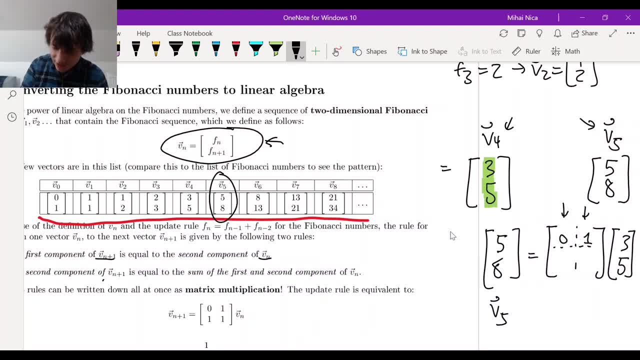 plus 1 copy of the 5 down here. So this is a 0, 1.. So that means take 0 copies of the first component and 1 copy of the second component. And the second number 8, is 1 copy of the 3. 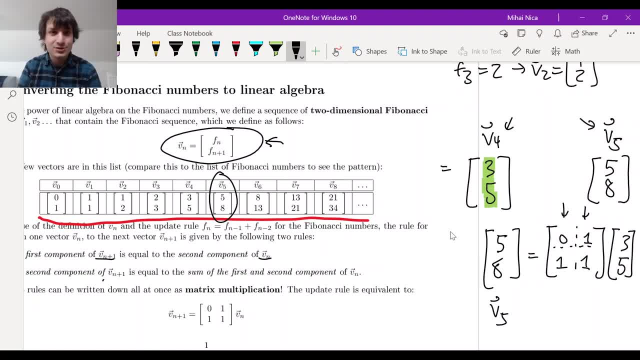 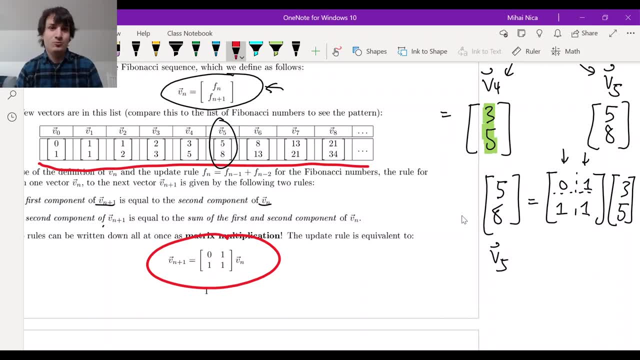 plus 1 copy of the 5.. So that's why it's a 1, 1 here And in general. what happens is you have this matrix multiplication rule, The Vs. they evolve according to this matrix: 0,, 1,, 1,, 1.. 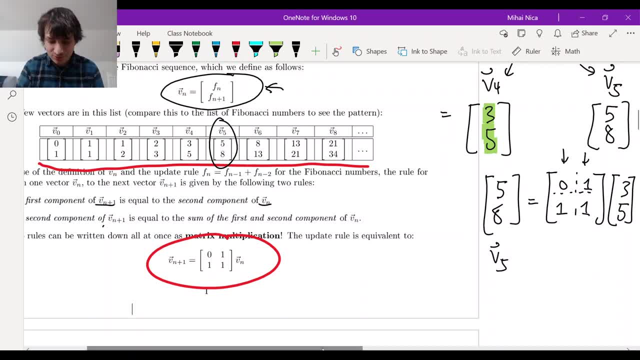 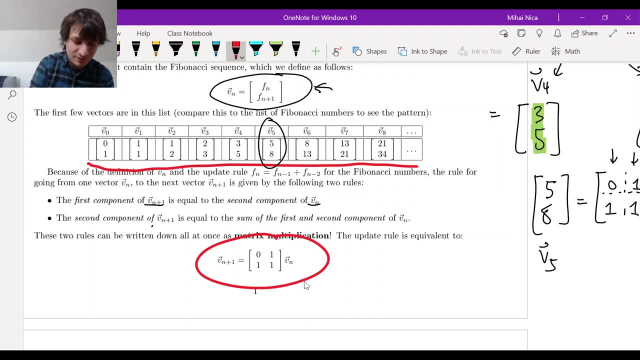 And 0,, 1,, 1, 1 is literally just an encoding of these two rules that we talked about, that the first component is equal to the second component of the previous vector and the second component of Vn plus 1. 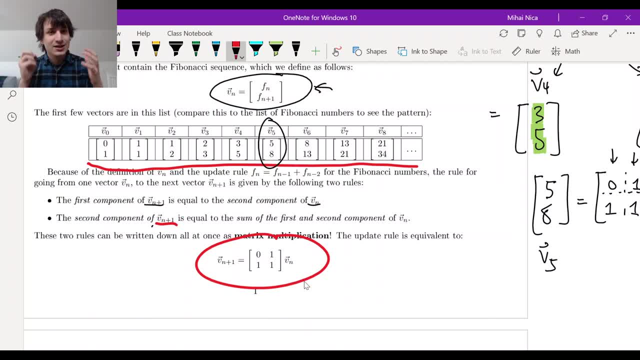 is equal to the sum of the first and second component in Vn. So that's what this matrix multiplication rule is doing. It's just taking what we know about the Fibonacci numbers and it's taking our definition of the vectors V and encoding it into a matrix multiplication. 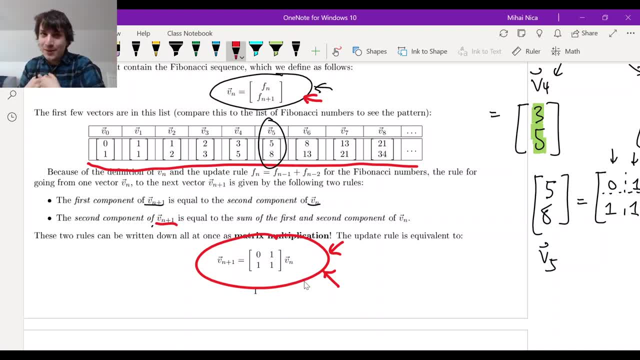 And now that we're in matrix multiplication land, now we're in business, we're going to be able to use all the rules you learned in linear algebra that were maybe painful at the time, and we'll see how they come out, to give us something nice about the Fibonacci numbers. 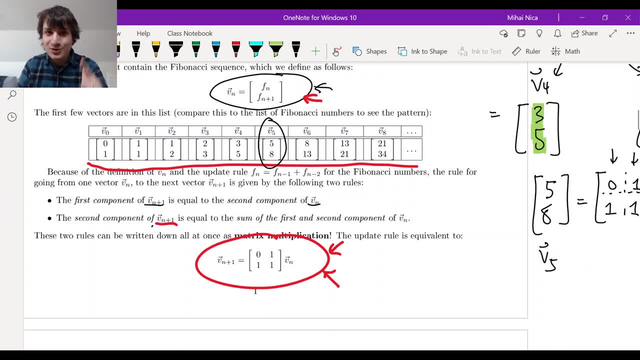 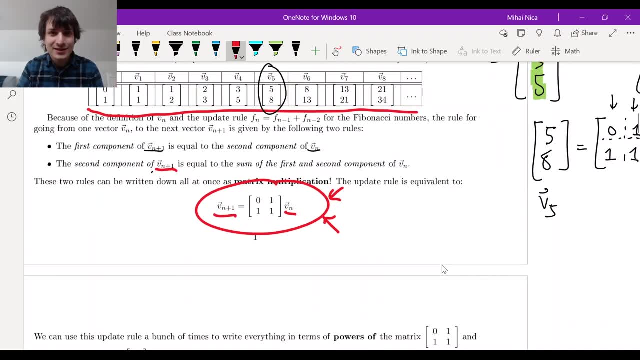 Okay, so this is the rule. Okay, first thing we're going to do right now. we still have a dependence: Vn plus 1 still depends on Vn, So let's get rid of that first of all. And the way you do that is you just apply this rule many times. 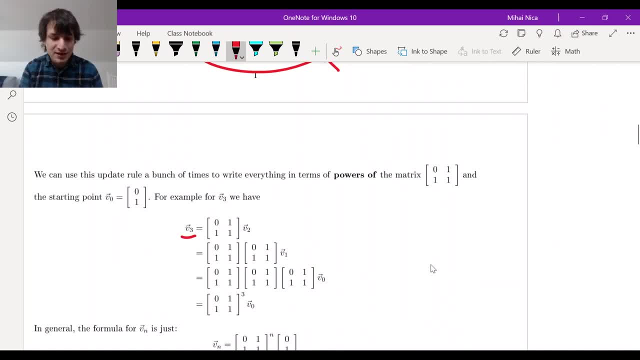 As an example, if you want to write V3, you could say: V3 is this matrix 0, 1, 1, 1 times V2.. Okay, but V2 itself is 0, 1,, 1, 1 times V1.. 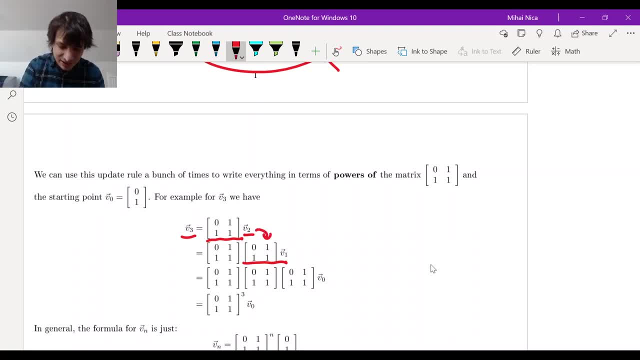 So that's what's going on here. We're replacing V2 by that, And V1 is itself 0, 1, 1, 1 times V0. And so you end up with, every time you do this, you end up with an extra copy of the matrix: 0, 1, 1, 1.. 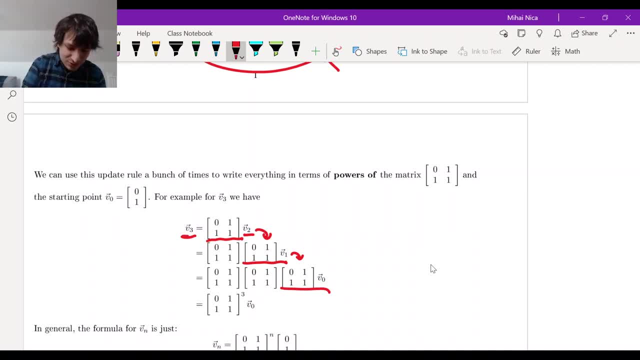 And if you do it n times, you end up that V3 is the matrix 0, 1, 1, 1 to the power, 3 times the vector V0.. And now you just remember, V0 was the very first thing on our list. 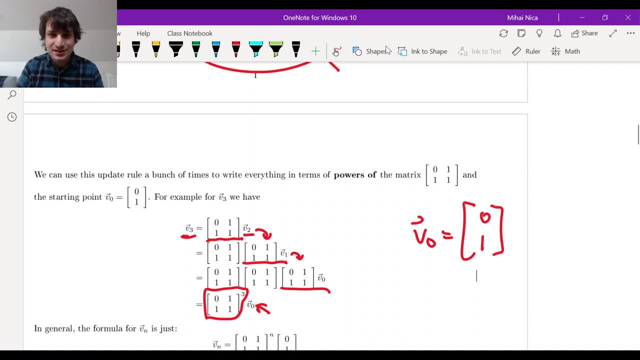 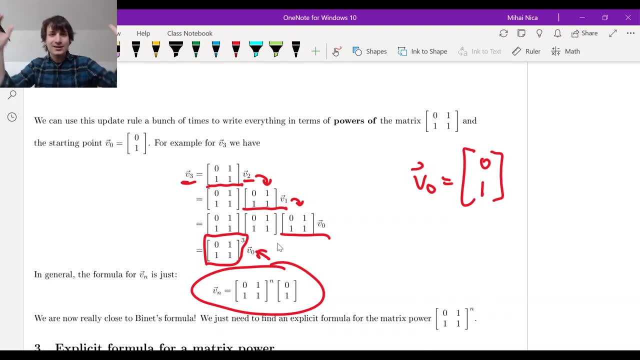 V0 was just 0, 1.. So what does this say? It just says, in general, the formula is like this: The nth item on the list is the matrix 0, 1, 1, 1 to the power n times 0, 1.. 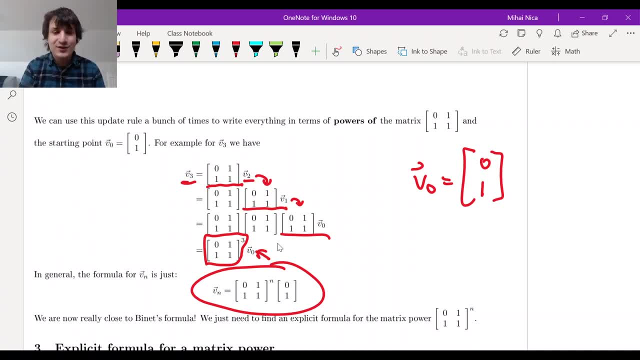 Okay, so you might think we've succeeded already. Now we have these Fibonacci vectors. They are written without any sort of dependence on each other. So the nth vector, Vn, just depends on the matrix power of this matrix: 0, 1, 1.. 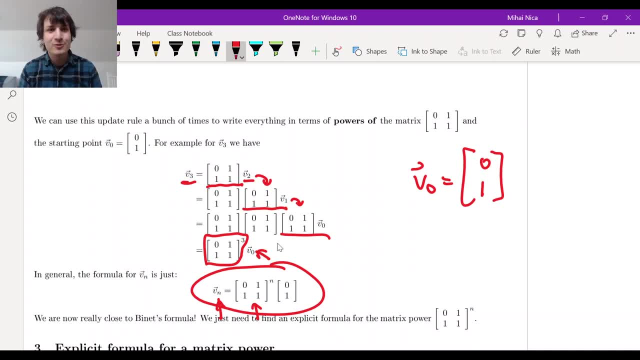 And if you saw this in linear algebra class, you might remember. there's ways to simplify matrix powers And if you use that, you'll get Binet's formula. So that's what we're going to do. on the rest of the video, 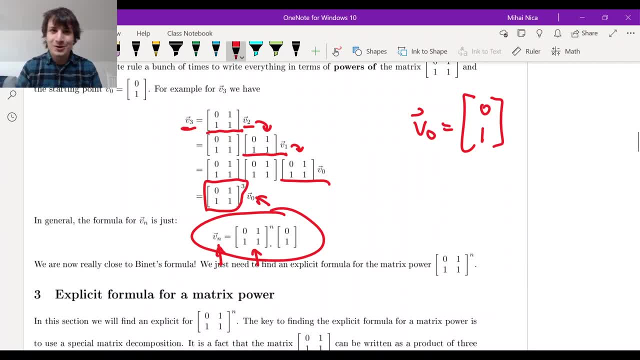 We're going to find an explicit formula for this matrix power. Okay, so here we go. That's what we're going to do now. We're going to find a formula for this thing and plug it in and see what we get. Okay, so here we go. 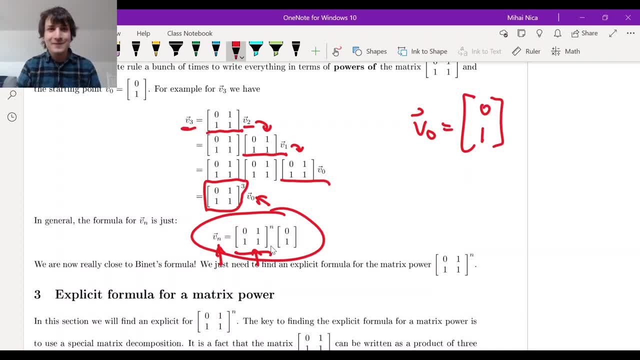 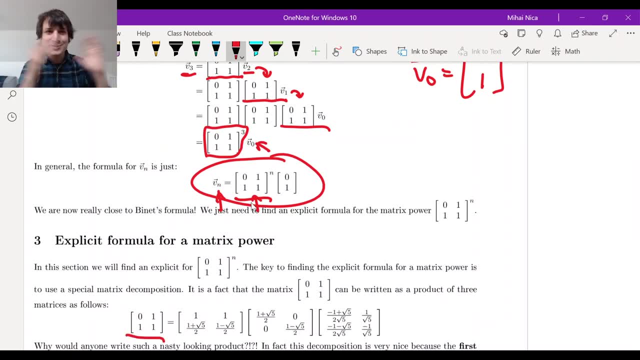 The key to this matrix power. this will seem like a total crazy thing if you've never seen something like this before. And the key is to write the matrix 0, 1, 1, 1, this nice matrix that only has zeros and ones in it. 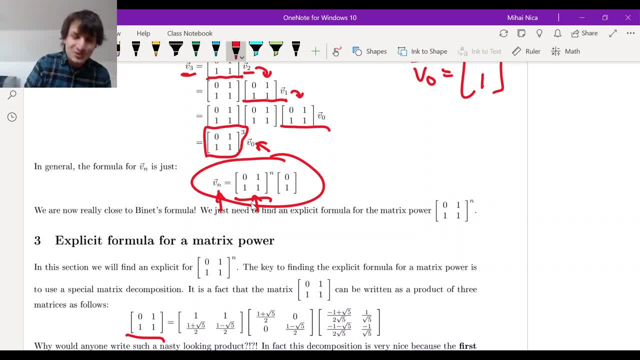 We're going to write it as a product of three matrices. So there's this funny matrix here: 1, 1, 1 plus square root of 5, 1 minus square root of 5 divided by 2.. That's a crazy looking matrix. 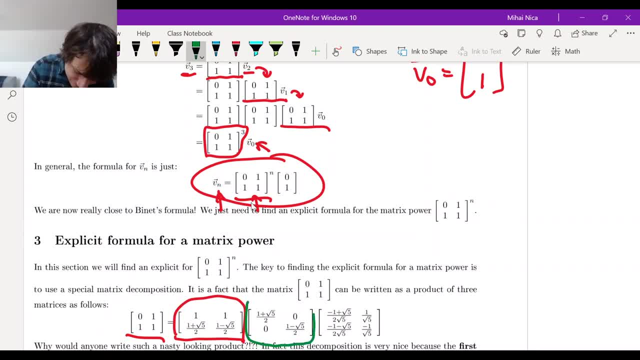 Then we have this matrix here in the middle: 1 plus square root of 5 divided by 2, 0, 0,, 1 minus square root of 5 divided by 2.. And lastly, the most ugly of the three matrices: 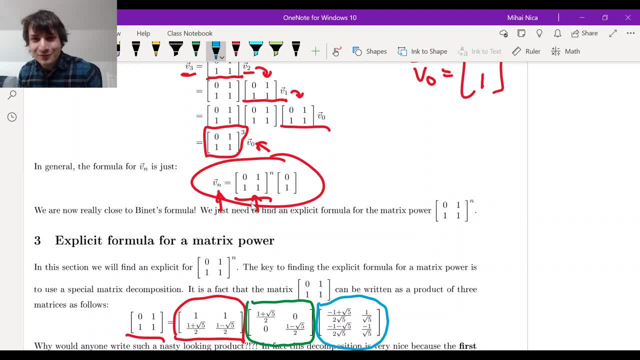 is this one over here: Minus 1 plus square root of 5, divided by 2 square root of 5, 1 divided by square root of 5.. Minus 1 minus square root of 5, divided by 2 square root of 5,. 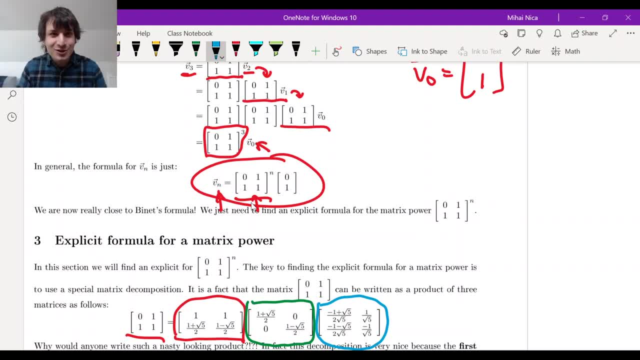 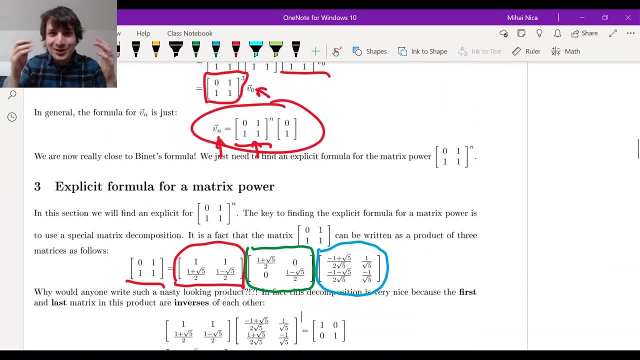 minus 1, divided by square root of 5.. Okay, and if I show you this, the first thing you should ask yourself is: why would anybody ever torture you with these crazy things? So we took a nice matrix. it was a totally reasonable matrix: 0, 1, 1, 1.. 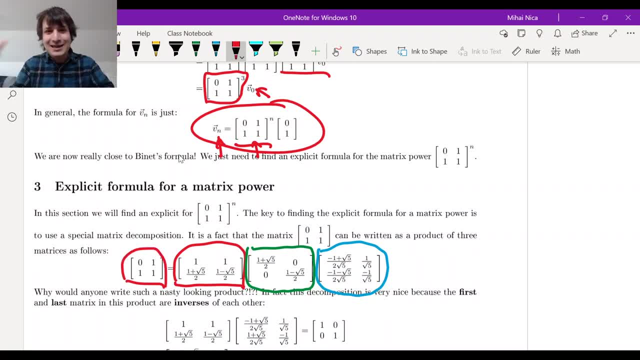 Okay, that's fine. And we wrote it as a product of three nasty matrices. Why would anybody ever do this? And it turns out these aren't just three arbitrary nasty matrices. they are very nice matrices, And the thing to notice is: 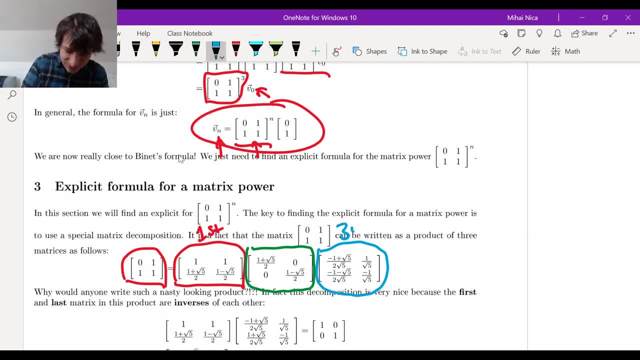 if you look at this first matrix and this third matrix. so the first matrix I circled in red and the third one is in blue. those two matrices, even though individually they look quite nasty, they are actually inverses of each other. 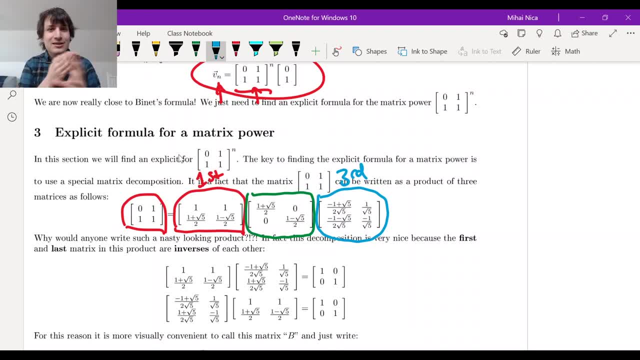 And what does that mean If you multiply them together in either order? so if you do the first one the first times the third, or you can do it the opposite way: you can do the third times the first when you multiply them together. 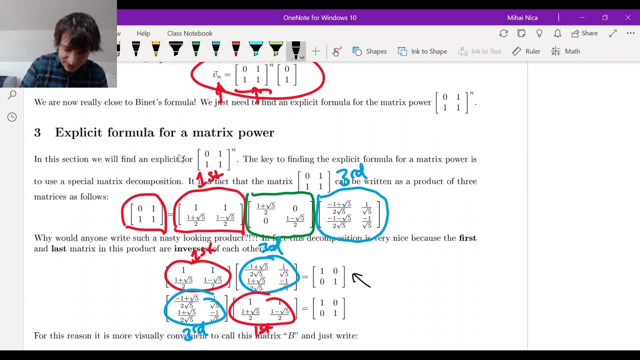 you get back to the identity matrix. This is the identity And this will be the key thing that makes everything work nicely. So the first and third matrix: they are individually very nasty, I admit, but they are inverses of each other. 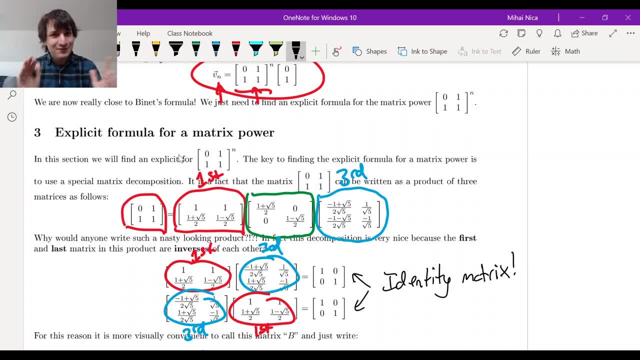 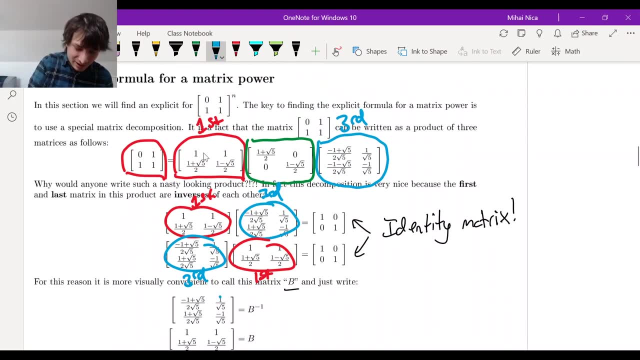 and that will make life easier for us in just a second. So they're inverses of each other. To make things a little easier to see, I'm just going to call this matrix B. So I'm going to call the third matrix B, inverse. 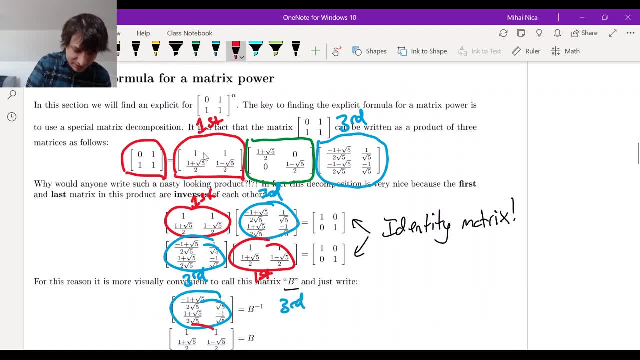 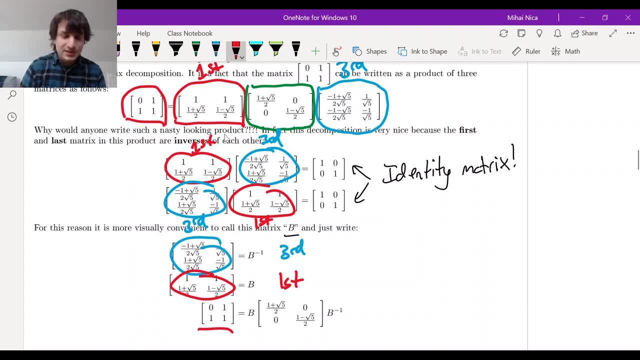 This is the third matrix And the first matrix. I'm going to call that B And they're inverses of each other. so they're B and B inverse. So what we did before was just writing this matrix: 0, 1, 1, 1. 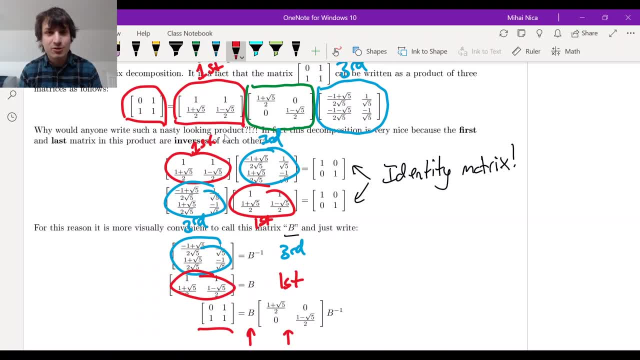 as B times this matrix, with 1 plus square root of 5 over 2 and 1 minus square root of 5 over 2 times B inverse. Okay, so if you call those B and B inverse now something nice happens. and it happens because B and B inverse are inverses. 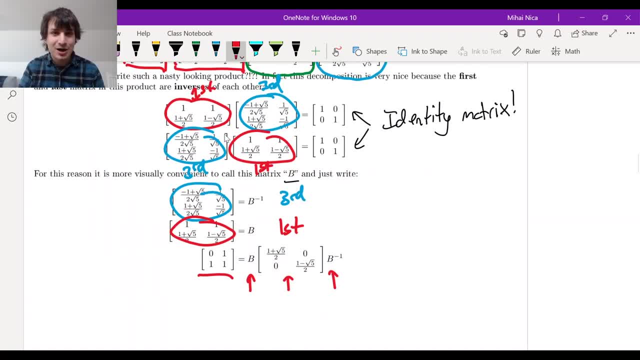 So let's see what happens when we do the second power of 0, 1, 1.. So let's do that here. So we're going to do the second power: 0, 1, 1, 1 squared. 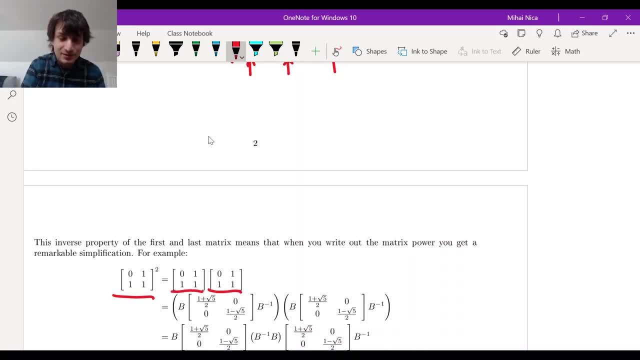 That's 0, 1 times 0, 1, 1, 1 times itself. So we're multiplying the matrix by itself And the matrix is B times this funny matrix times B inverse, and I'll just plug that in. 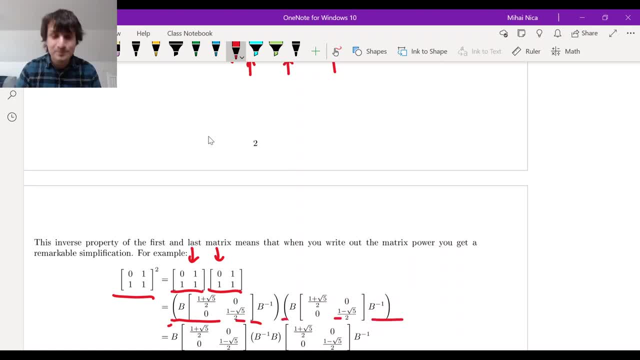 And when you plug that in, so you've got three matrices here and you've got three matrices here, and if you regroup the terms, the cool thing that happens and this is like the miracle. this is the miracle of the piece. 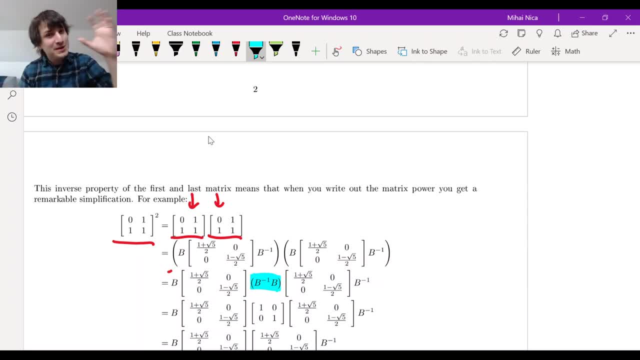 is this thing. right here You end up in the middle. you have a B inverse times a B. So you have the B inverse from the first term, you have the B from the second term and they're right next to each other. 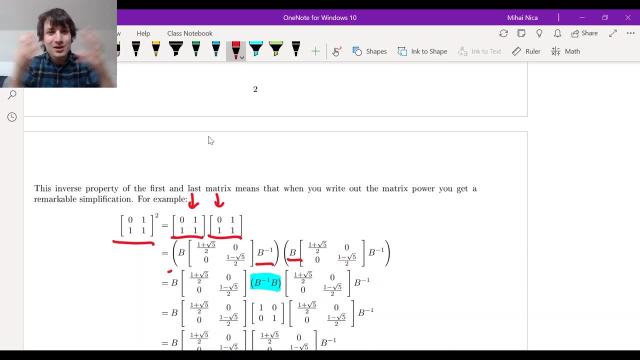 And B inverse, and B are inverses of each other. so when you multiply them together you get the identity matrix. And so on the next line, I've replaced it with the identity matrix, And multiplying by the identity is like multiplying by 1.. 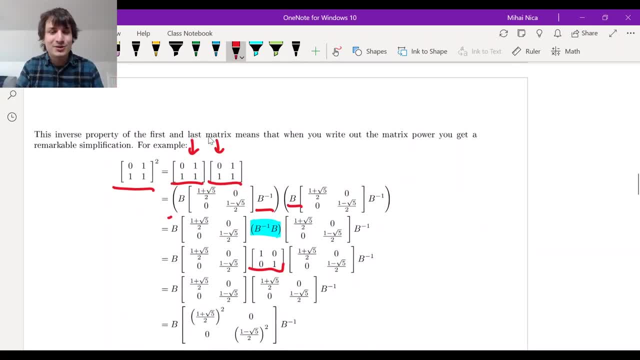 So that doesn't do anything. It's like multiplying by the number 1.. So sort of this funny looking thing in the middle. it got simplified because it was an inverse of itself, And that is a really nice property. When you do that, then you end up with two copies of this diagonal matrix. 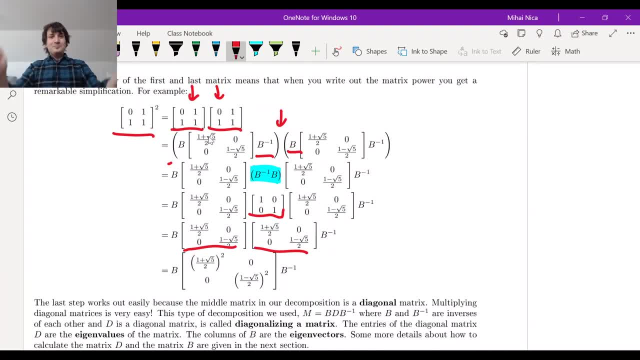 multiplying each other in the middle. Okay, and now you see the next beautiful thing. So far I've said that B and B inverse, being inverses of each other, was important. The middle matrix, the second term in our decomposition, that was a diagonal matrix. 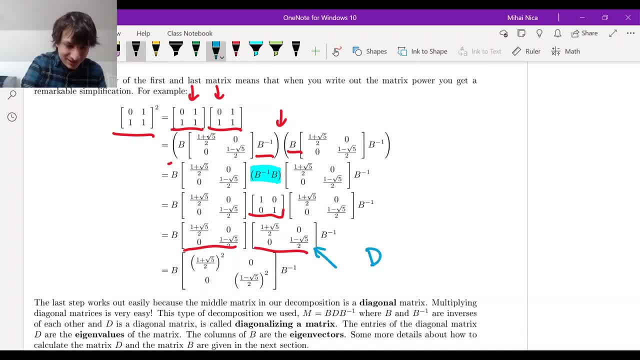 So this is a diagonal matrix. I think I did it in green, Let's keep this guy in green. So this matrix over here, the middle matrix, this is a diagonal matrix. Okay, and why is that so nice When you multiply diagonal matrices? 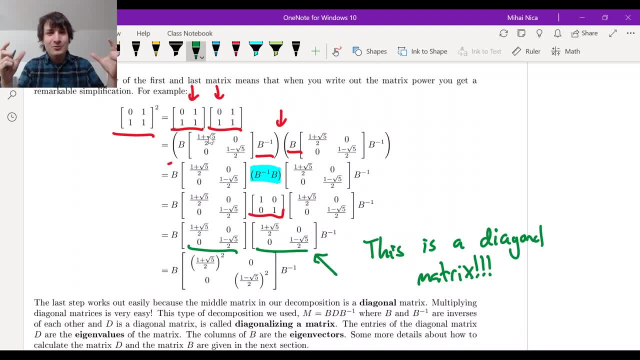 the multiplication is very easy. So normally when you multiply matrices you have to do row by column. It's like a big mess. It's like the size of the matrix squared additions and multiplications. So that is a lot of work. But for diagonal matrices 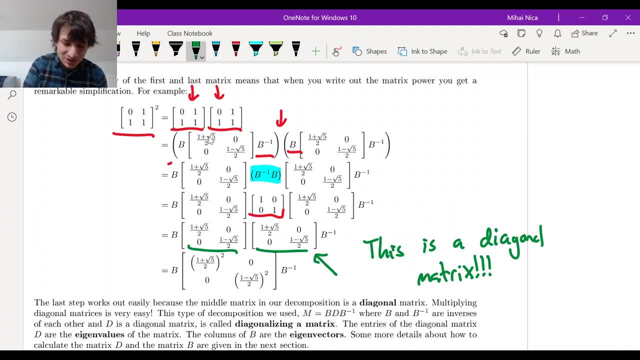 the diagonal terms multiply each other and they sort of don't talk to the other diagonal terms. So when you multiply this by this on the next row you get a diagonal matrix and you only have to multiply the diagonal terms. It's very simple. 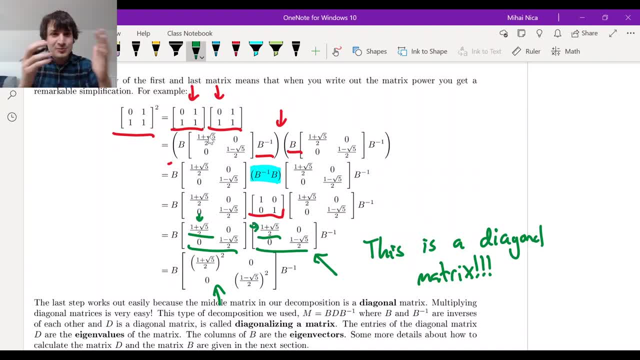 So this was a 1 plus square root of 5 over 2.. This was a 1 plus square root of 5 over 2.. They multiply together. you get a 1 plus square root of 5 over 2 squared. 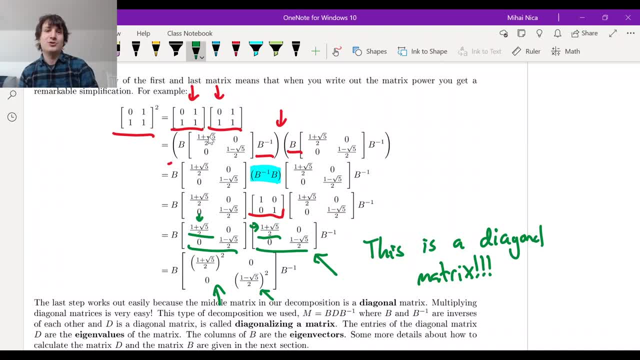 Similarly in the other diagonal entry down here you have a 1 minus square root of 5 over 2 squared. So beautiful thing. We've simplified multiplying the matrices Because of this crazy cancellation with the B and the B inverse. 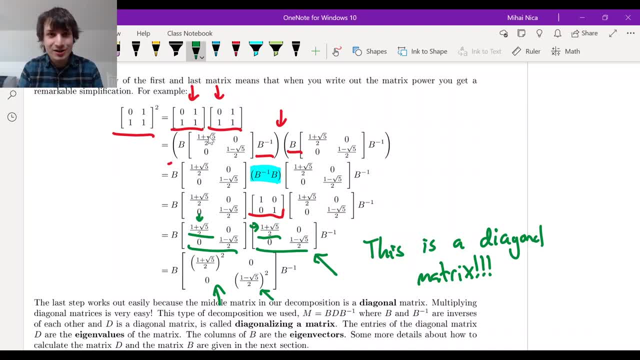 we ended up multiplying diagonal matrices, and that is much easier. You just take powers of the diagonals, So multiplying diagonal matrices is really easy, and this is why this sort of simplification works. Okay, so to summarize what we've done so far, 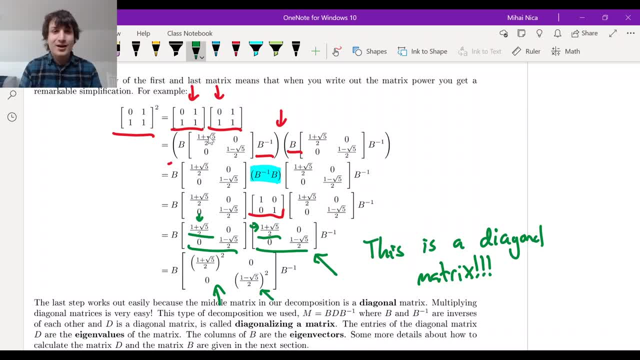 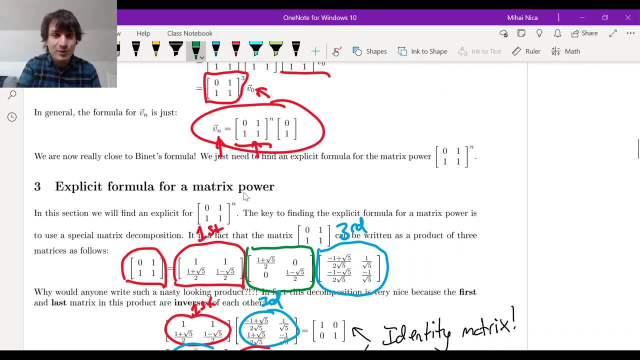 we've really taken advantage of two things. One is that when we wrote our matrix, a period of time here when we did this decomposition- the first matrix and the third matrix, the red matrix and the blue matrix, and this- those were inverses of each other. 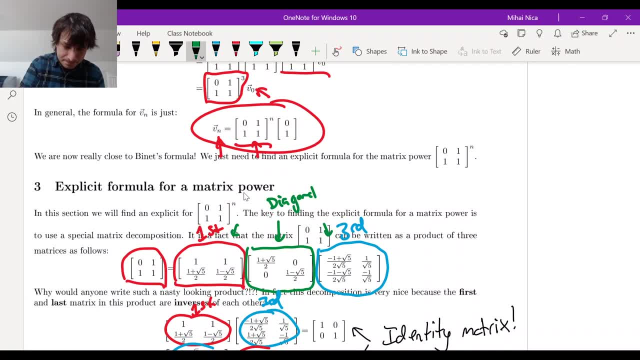 and the middle matrix is diagonal. So this is the second matrix, this is the diagonal matrix, And this is called the eigenvalue, eigenvector, decomposition of the matrix or diagonalizing the matrix, And this is something you might have learned in linear algebra. 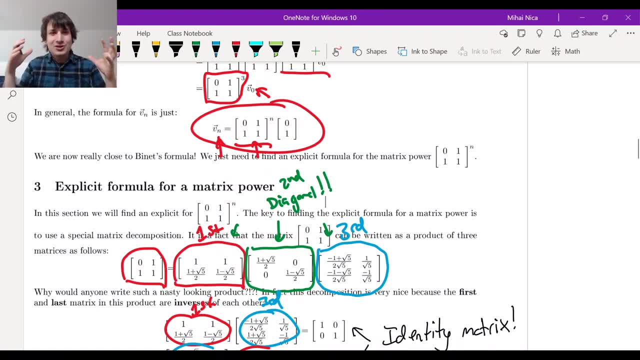 or maybe you've never seen before and it is a cool way to simplify matrix multiplication. So this kind of thing, how you turn any matrix into this kind of product of inverses of each other with a diagonal in the middle, that is called diagonalizing a matrix. 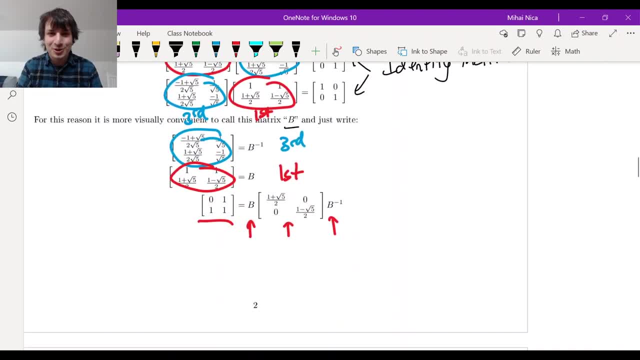 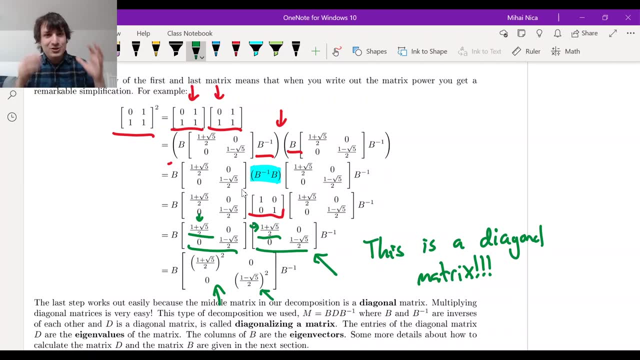 and it makes these kinds of computations easier. Okay, so I have a little blurb about this here. Yeah, so this is called diagonalizing a matrix. The numbers on the diagonal matrix in the middle, those are called the eigenvalues of the matrix. 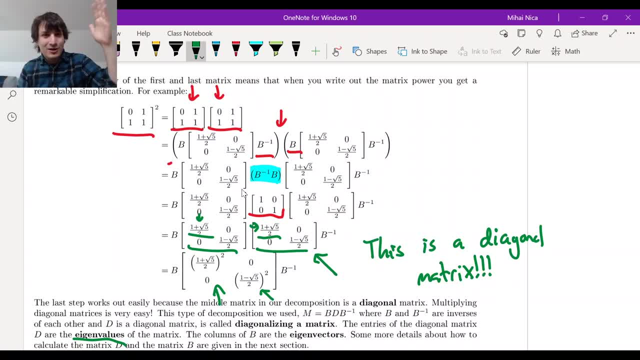 and the rows and columns of the, the columns, rather, of the matrices. on the outside. those are called the eigenvectors, And you can learn a lot about eigenvectors and eigenvalues. I'm not going to go into a huge amount of detail here. 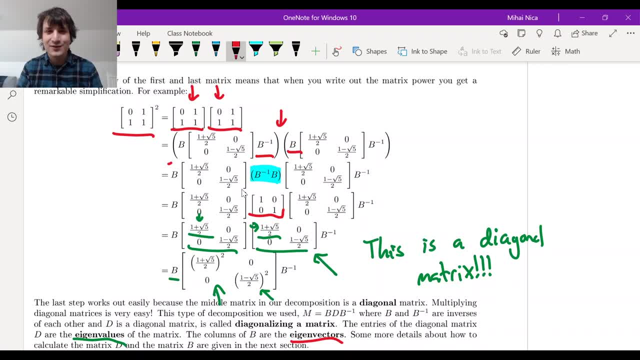 I do have a little section at the end where I calculate the eigenvectors and eigenvalues. So if you're wondering, okay, this is all very nice, but where the hell did this come from? The answer will be in that last little section. 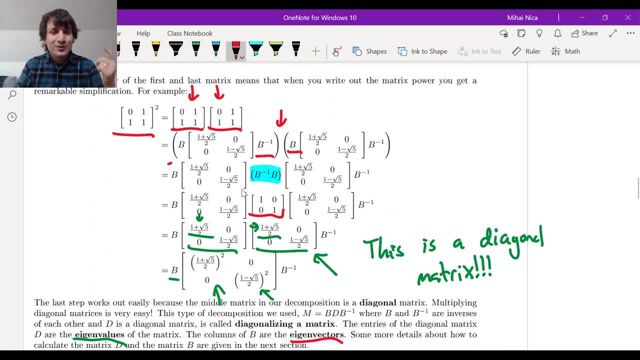 But for now we have this nice trick for computing powers And I did it so far. I only did it with the second power, so 0111 squared, But let's do it in general. Let's do 0111 to the power n. 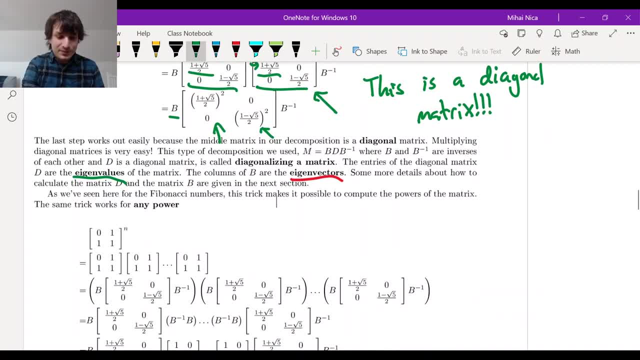 And the same kind of trick works. So first thing you do take 0111 to the power n. that's a product of the matrix times, itself n times, And in each of those instances write the matrix as the diagonalization. 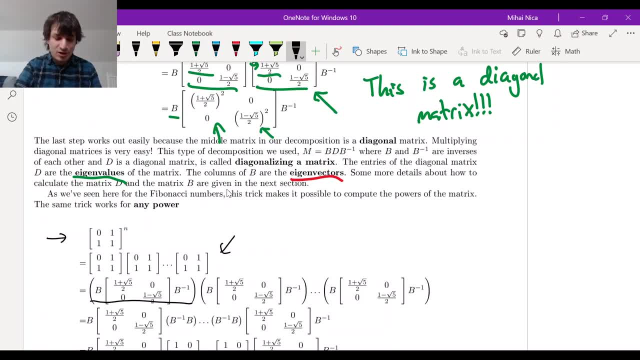 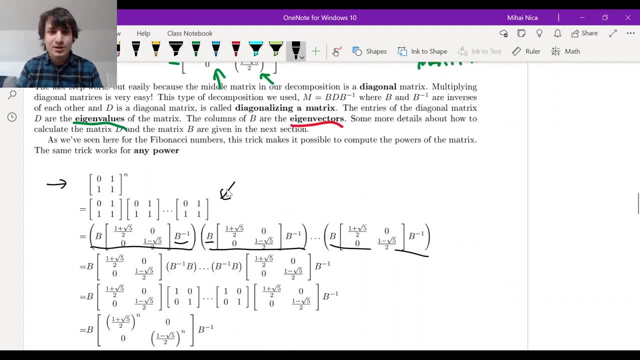 b times the diagonal matrix, times b inverse. do that for all of your copies. And now in between you notice that b inverse and b are appearing right next to each other. So if you group the b inverses and the b's together, 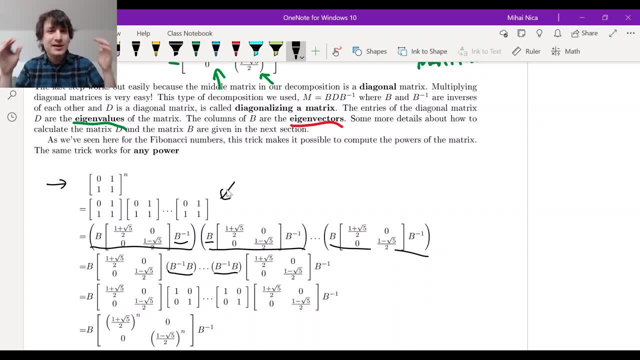 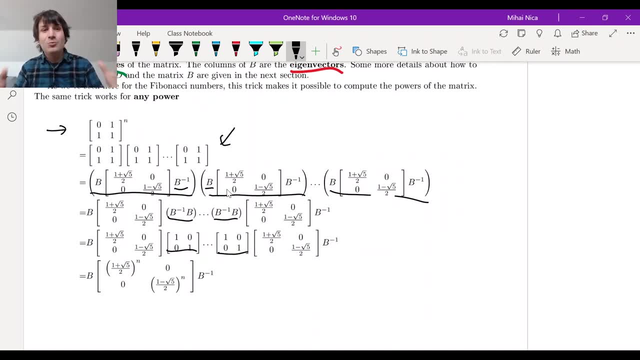 that will simplify a lot of terms inside the middle of your product. And that's because b inverse times b is always the identity, So it's simplified quite a lot. You have all these identities in there. When you multiply by the identity, that's like doing nothing. 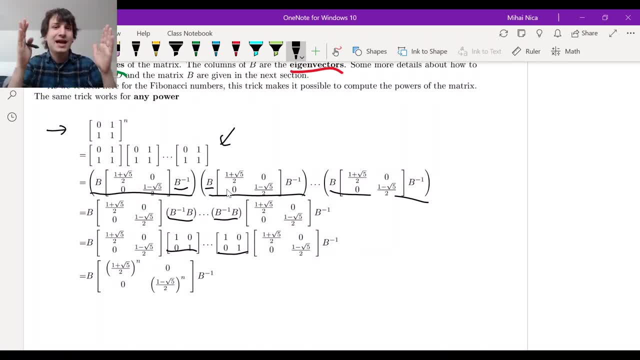 So what you're left with is a product of a bunch of diagonal matrices. You have n copies of the diagonal matrix 1 plus square root of 5 over 2, 1 minus square root of 5 over 2, in the middle of this big product. 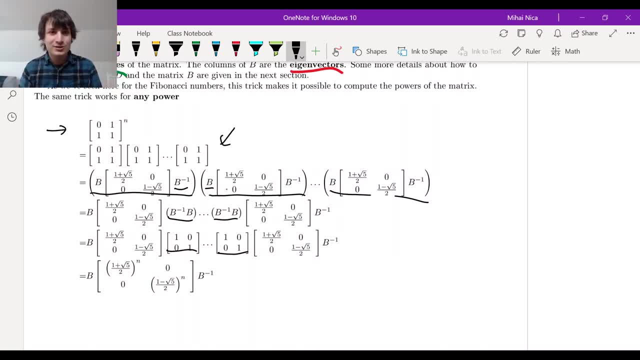 And multiplying diagonal matrices is easy. All you do is multiply the individual diagonals, so you end up with this thing: 1 plus square root of 5 over 2 to the power n because there's n copies. because there's n copies. 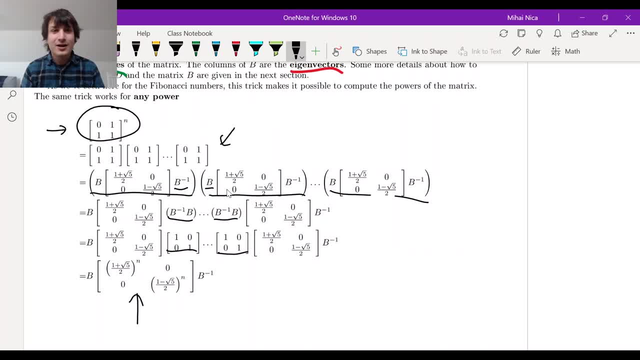 So there's a nice way to convert this power of this matrix into something very explicit without having to do a huge amount of computation to figure out what's going on. So we're very close to the end here And that is because, remember, we had this formula: 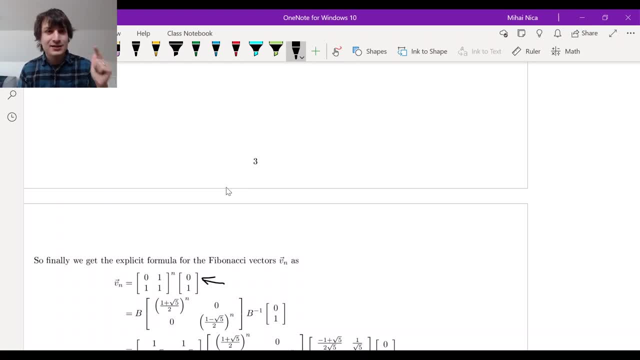 that vn was 0, 1, 1, 1 to the power n times 0, 1.. If you plug in what we just did, that is this matrix: b times this thing to the power n times b inverse. We had formulas for b and b inverse. 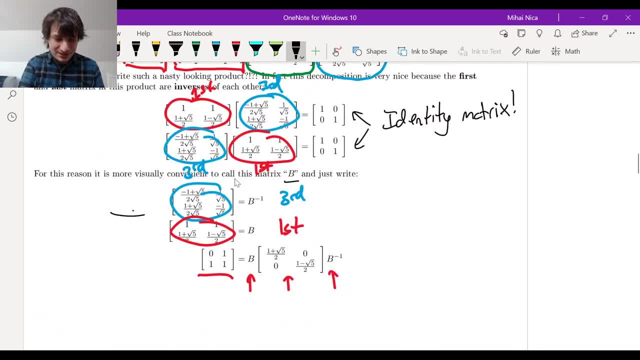 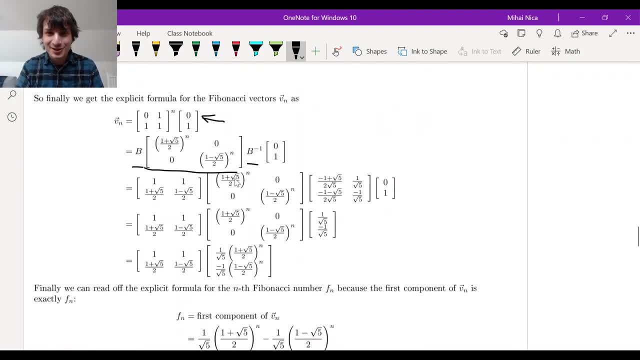 We had these nasty matrices over here, So that was this definition. If you plug those in, what do you get? You get this formula. So I've plugged in what b and b inverse are And I've plugged in also that v0. 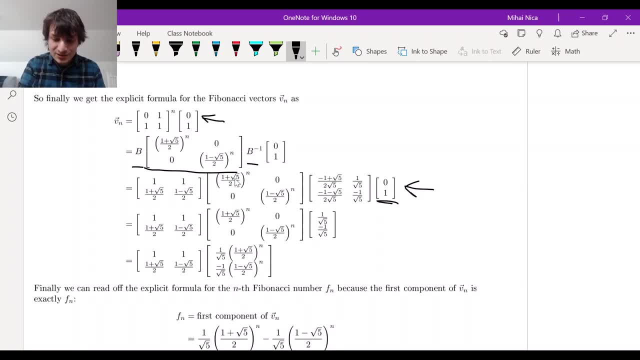 was 0, 1.. So if you start doing a little bit of multiplication, so this is a nasty matrix times 0, 1.. 0, 1 just means look at the second column. So even though the first column is quite nasty, 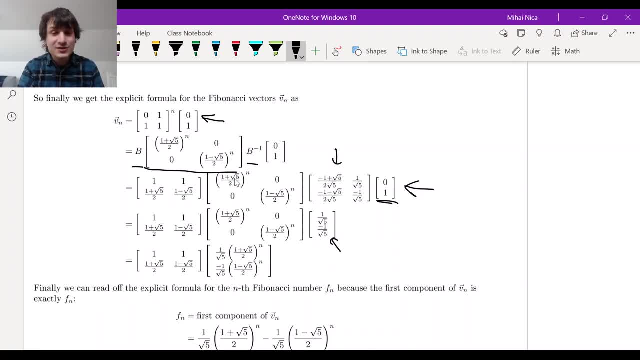 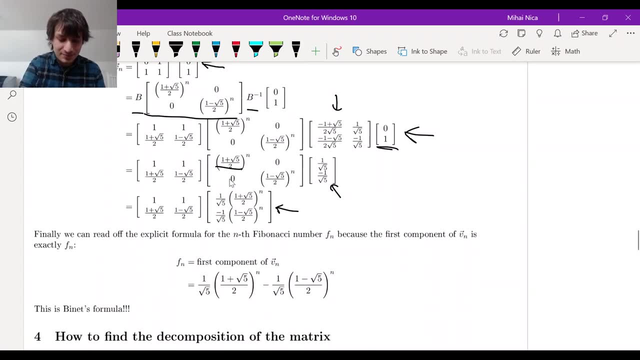 we only end up with the second column here. So when you multiply this vector times a diagonal matrix, that's also quite nice. So you end up with this. So the first component multiplies the first component, The second component multiplies the second component. 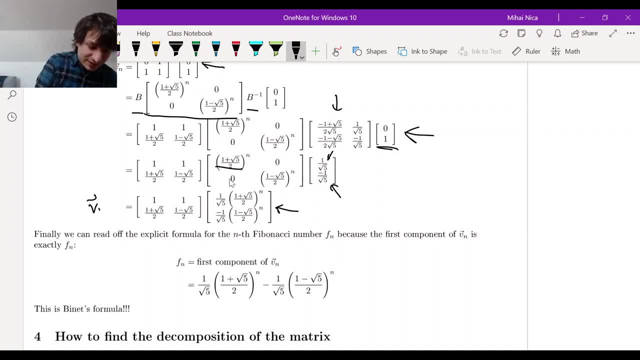 You end up with this thing. So this is the formula for the vector vn. It is this funny matrix: 1, 1.. 1 plus square root of 5 over 2.. 1 minus square root of 5 over 2. 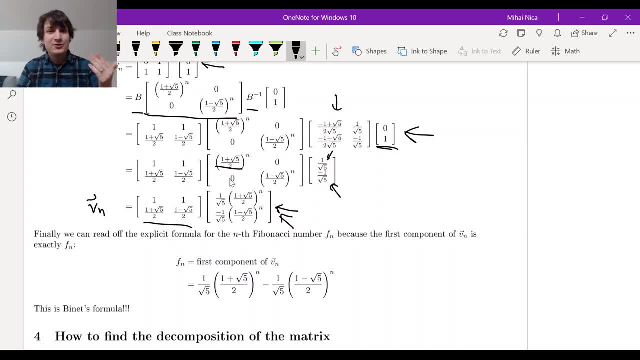 times this vector which involves powers of n, That's the vector vn. This is the original question we wanted to ask. We wanted to know what is a formula for the Fibonacci numbers And the Fibonacci numbers. remember, vn was defined to be fn, fn plus 1.. 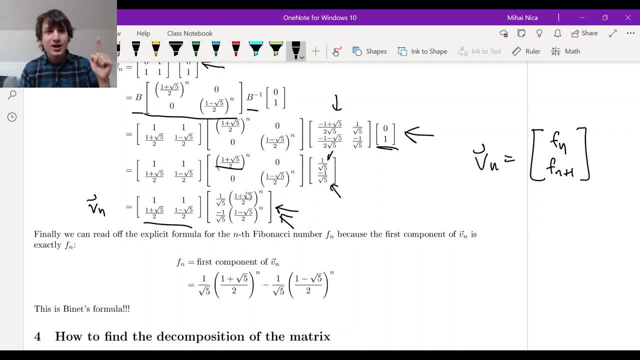 So if we want to know what is fn, the nth Fibonacci number, all we have to do is look at the first component of vn. So we're going to look at the first component of vn, And the first component of vn is this product: 1,, 1,. 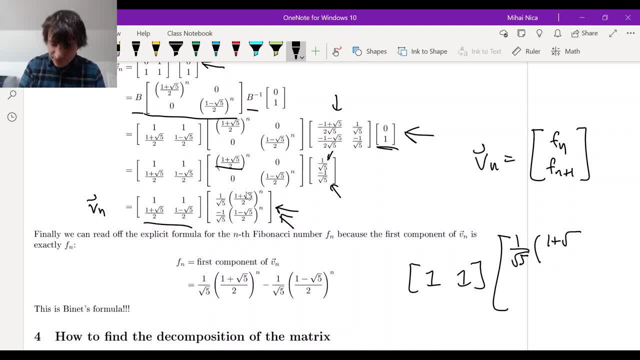 times this thing: 1 divided by square root of 5.. 1 minus square root of 5 over 2. to the power n. 1 divided by square root of 5.. 1 minus square root of 5 over 2. 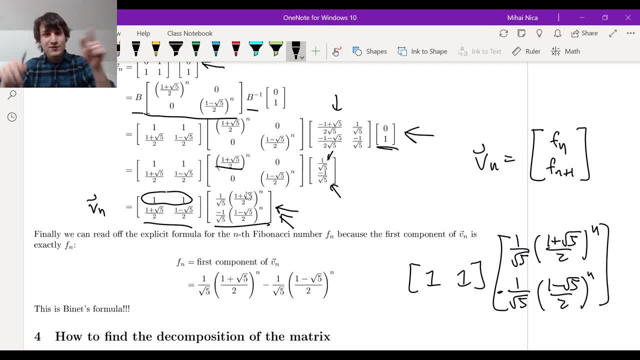 to the power n with a minus. So that was this vector And we're looking at the first row of this matrix. And if you multiply those out, 1, 1 means add them together: 1 times the first term, 1 times the second term. 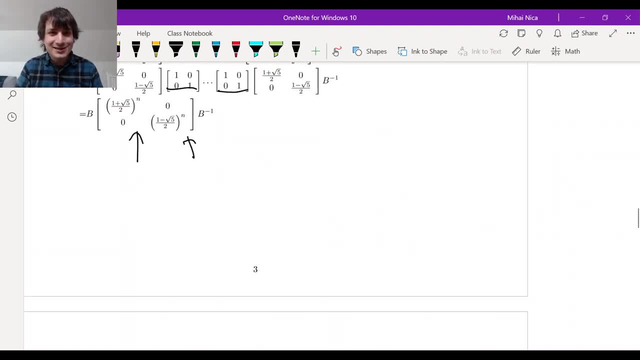 And you end up exactly with Binet's formula. So that is an explanation of how Binet's formula works, And it came from this crazy decomposition of the matrix 0, 1,, 1,, 1.. And if you look at the diagonal of the matrix, 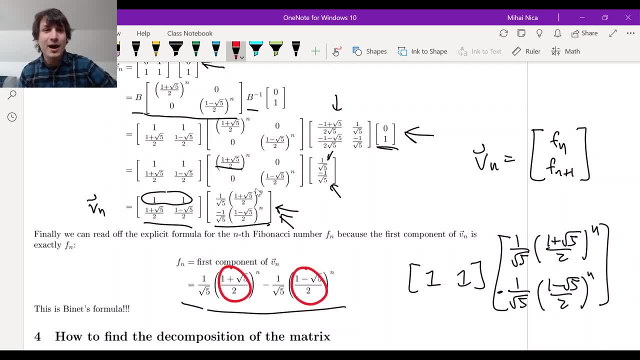 those are these two numbers: 1 plus square root of 5 over 2 and 1 minus square root of 5 over 2.. Those are the eigenvalues of the matrix. And there's some funny work. Where did these numbers come from? 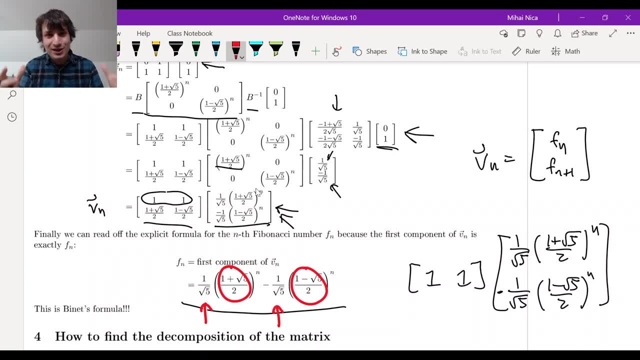 Those came somehow from the eigenvectors of the matrix. But in general for any matrix or any kind of rule you have for a linear combination of the previous terms in the sequence giving the next terms in the sequence, you can always do this kind of thing. 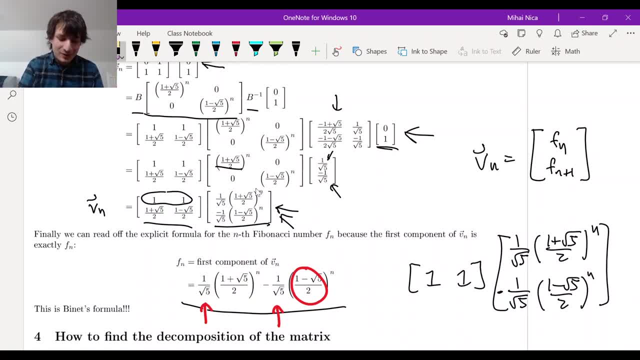 and you're always going to end up with some eigenvectors and eigenvalues. So this is a cool application of linear algebra. I remember when I was learning linear algebra I really hated it, But stuff like this makes me think that maybe it was worth it. 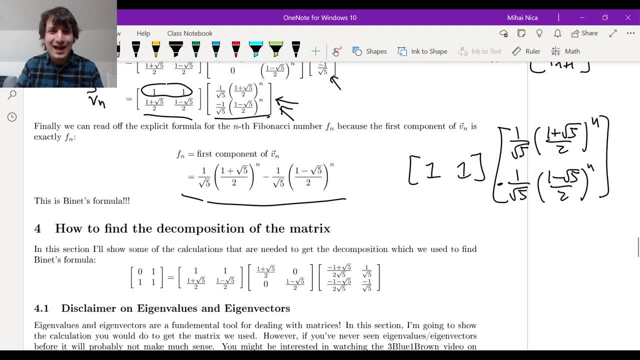 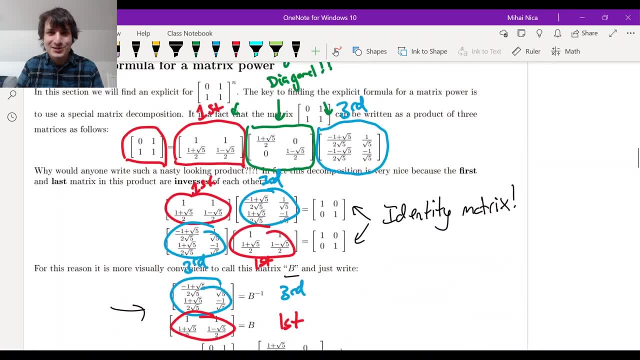 If you are interested in the next section here I have some calculations on how I calculated these numbers. So in this part of the presentation here I said: look, you just do it and you get this magical thing And in fact what you spend a lot of time.